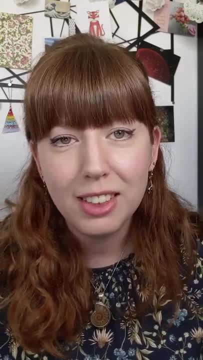 there's still a one in a thousand chance that this could just be a statistical variation in the data. So the LHCb collaboration has been successful. It has a bit more work to do before they can start celebrating. 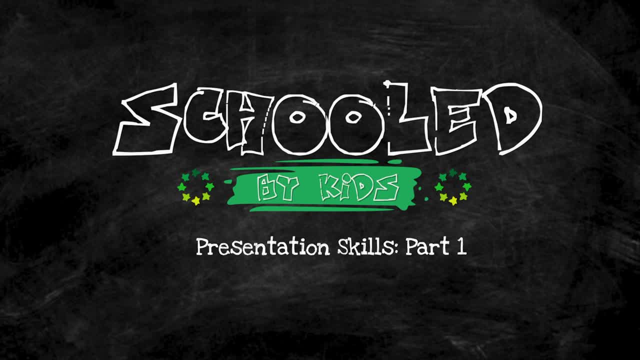 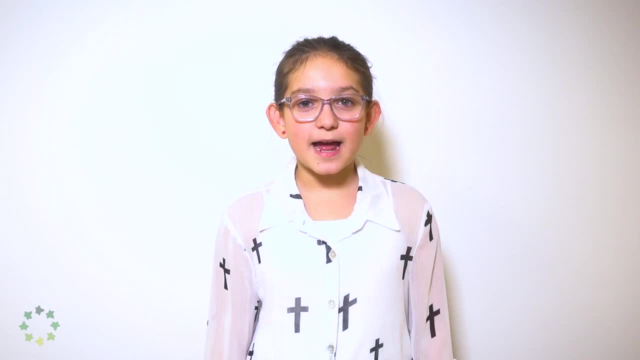 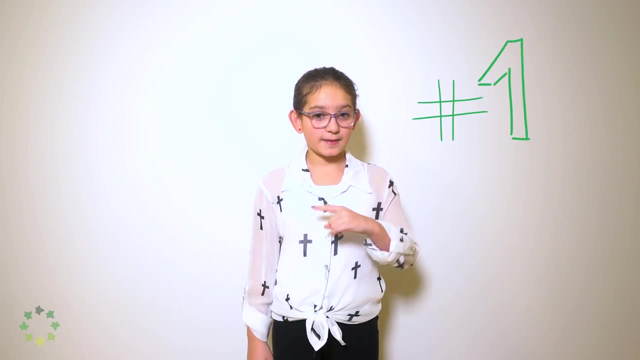 School: My kids Presentation skills, part one. My name is Kenna And I'm going to teach you how to do a great presentation. It's my version of a TED talk. Number one entrance: When you walk in, you have to be confident. 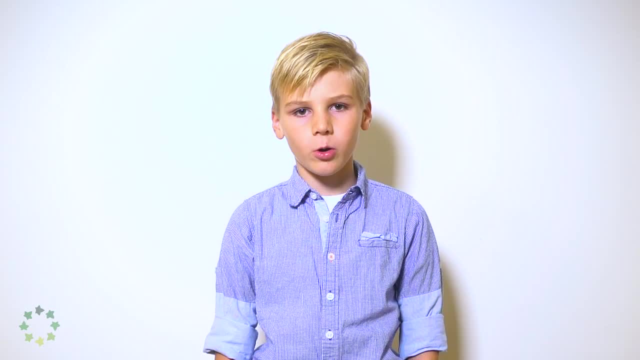 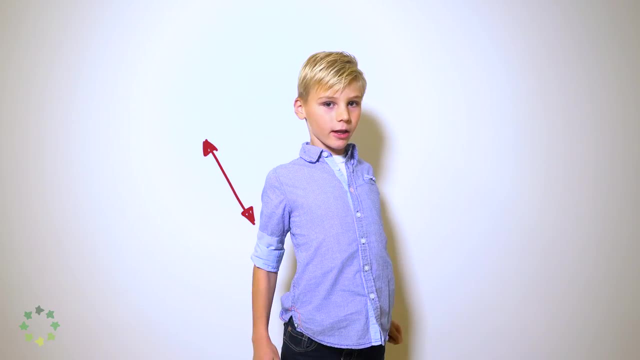 Smile. If you don't smile, the audience is going to be like what: You have to walk in confidently. You should have your shoulders back, but not like all the way back. Don't move around so much, because that's a little bit distracting. 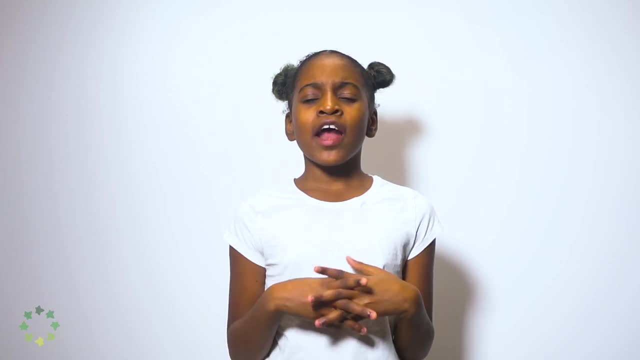 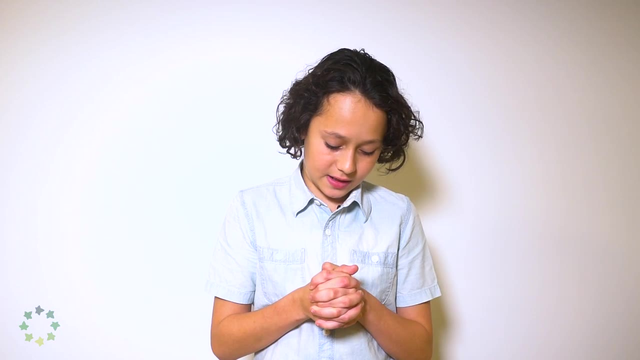 Because then the audience is going to lose attention. If you're having a little bit of trouble putting your hands by your side, you can put your hands above your belly button. This is a very good speaking stance that I actually use a lot. Here's the most important part. 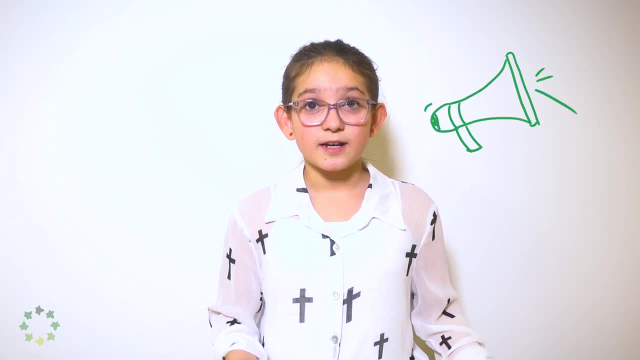 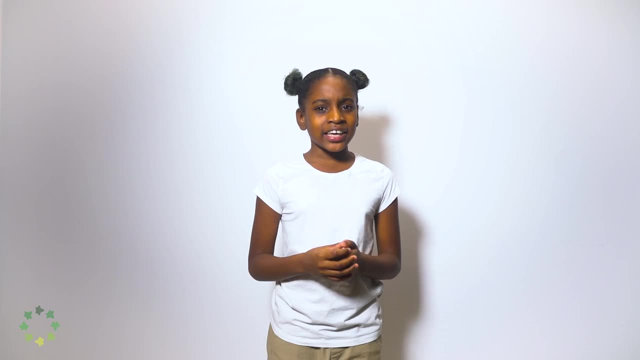 Introduction. You need to get these people's attention in ten seconds Because that's it: Ten seconds To get your audience's attention. If you don't use that ten seconds, everybody's going to start being bored. If I start with a hook, they tend to stay more engaged. 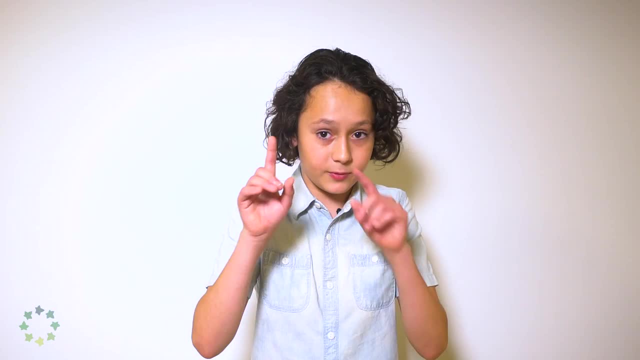 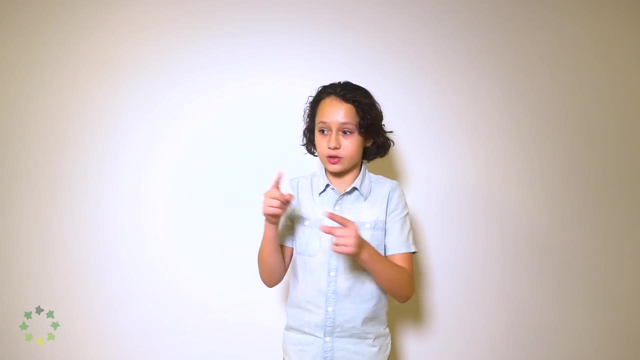 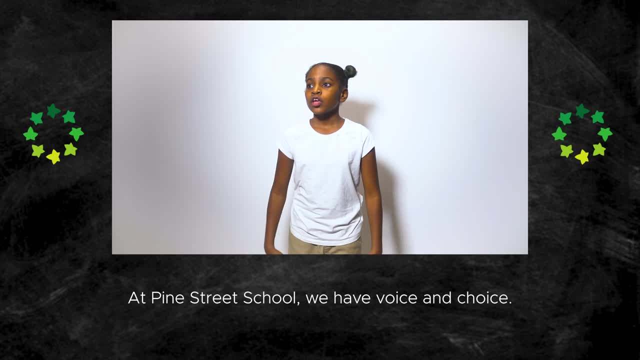 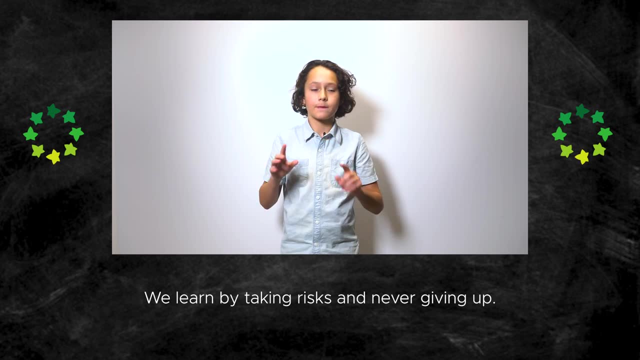